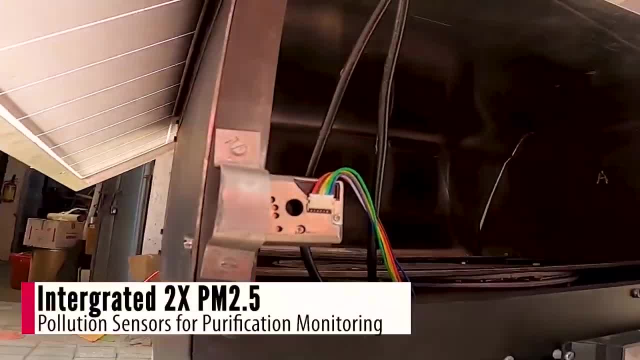 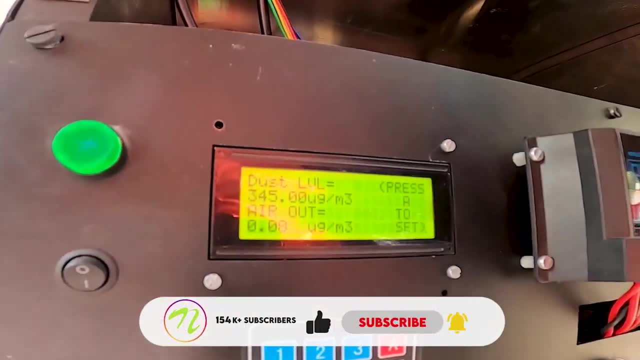 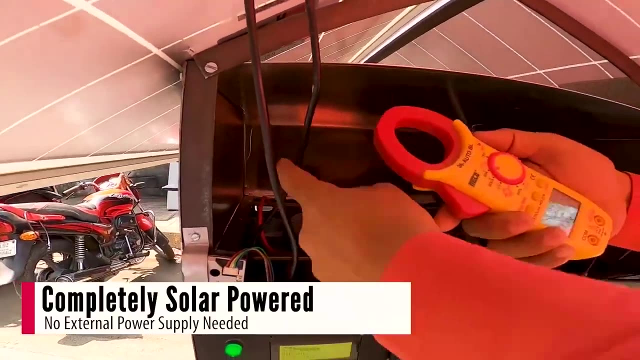 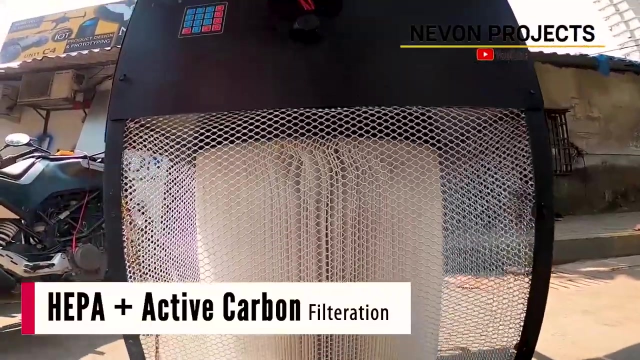 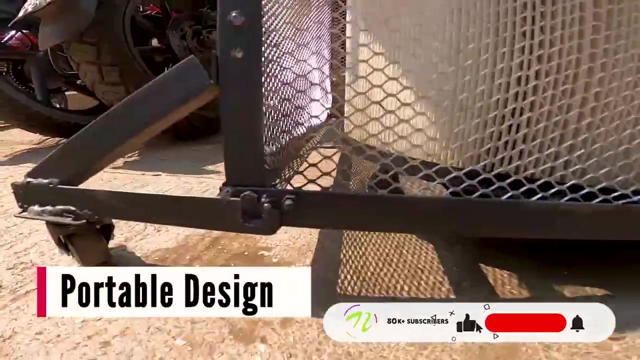 and improving the AQI. AQI is designed to integrate a system of micro-emissions in both both wind and air to create an isolated system of the power of the air. All these systems require 48% of the AQI, equal to 25% of the total. AQI is a completely new technology that is making it possible to control and manage water in the atmosphere without causing warming and the potential for a cold. I think the electricity generation is currently our biggest asset, especially in the global climate. We have the power to do everything we can and bulbs. 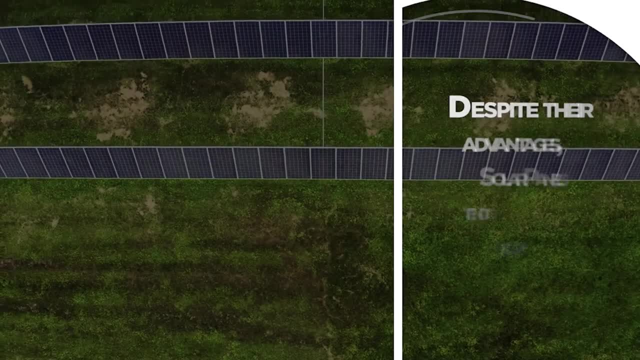 We are the only one that can do everything we can, and we are the only one that can do everything we can, and we are the only one that can do everything we can, and we are the only one that can do everything we can. Solar footpath. Despite their advantages, solar panels tend to occupy a lot of space. 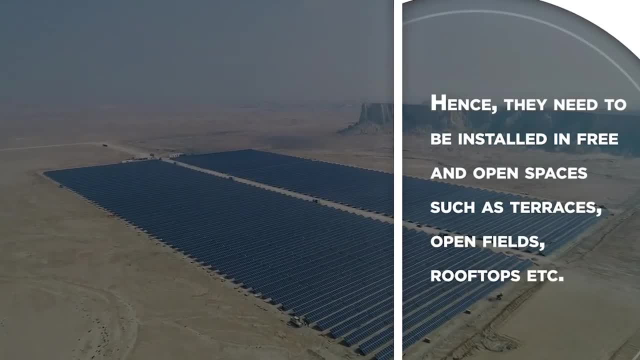 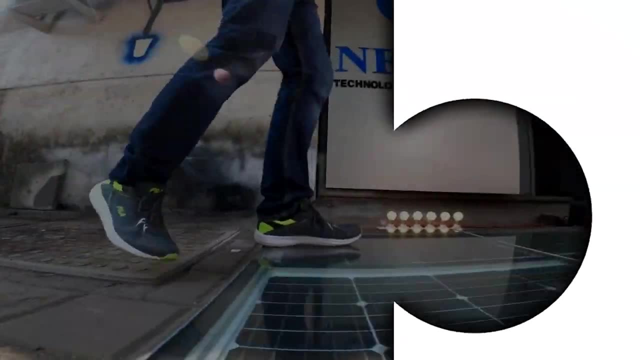 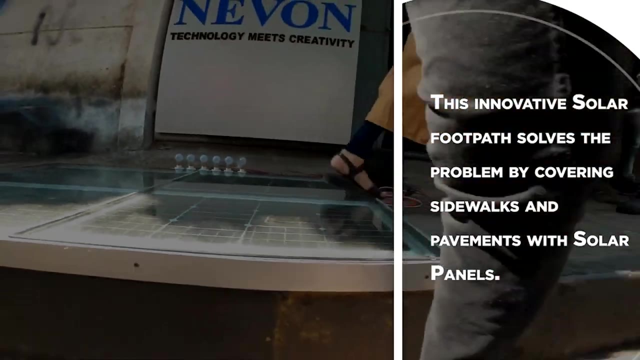 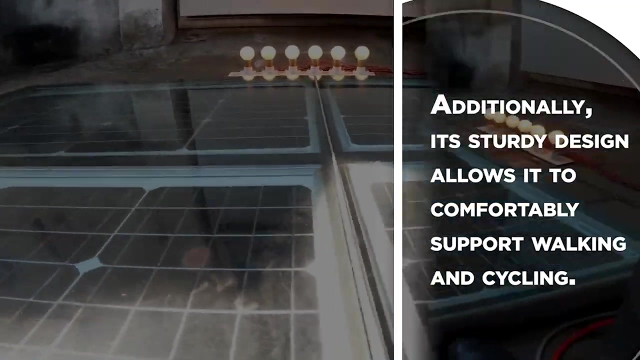 Hence they need to be installed in free and open spaces, such as terraces, open fields, rooftops, etc. So this innovative solar footpath solves the problem by covering sidewalks and pavements with solar panels. Additionally, its sturdy design allows it to comfortably support walking and cycling. 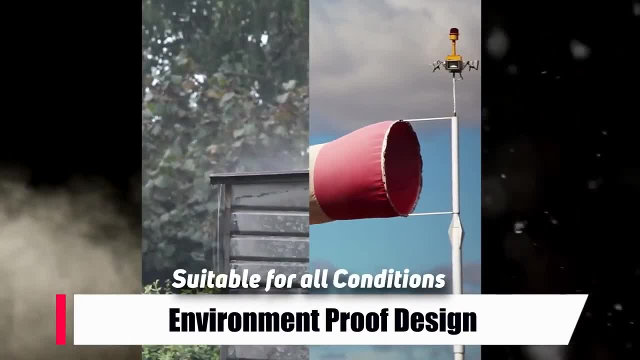 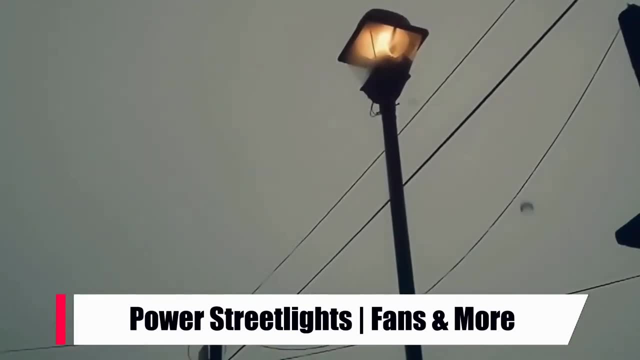 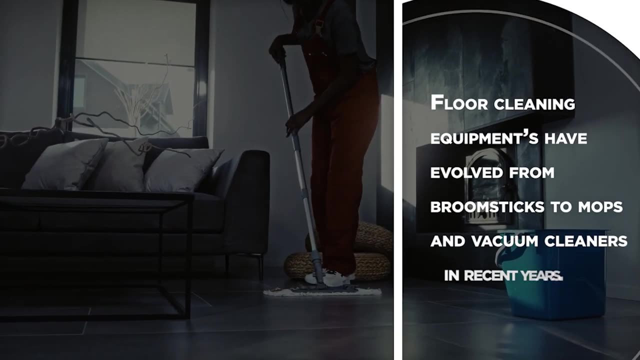 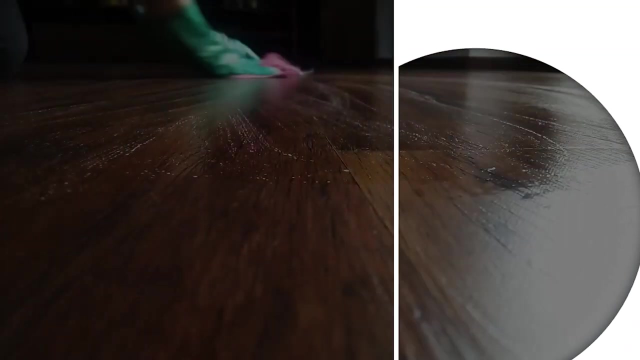 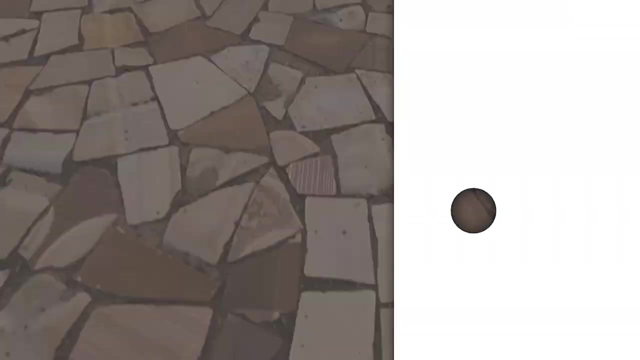 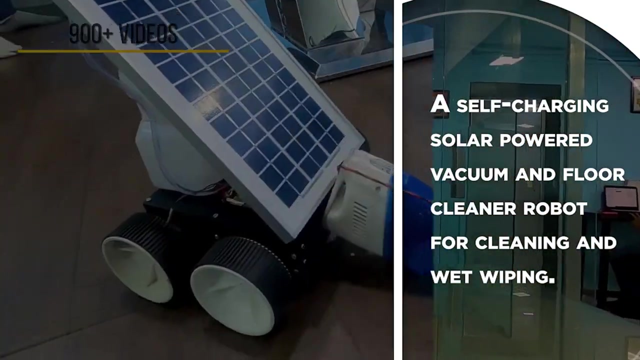 Solar Floor Cleaner. Floor cleaning equipments have evolved from broomsticks to mops and vacuum cleaners in recent years. Well, this innovation takes it to the next level by making the process fully accessible. So a self-charging, solar-powered vacuum and floor cleaner robot for cleaning and wet wiping. 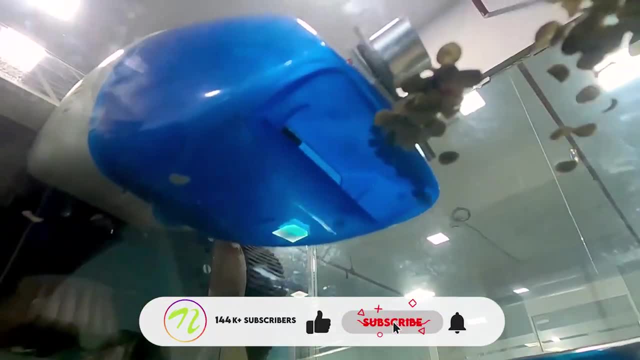 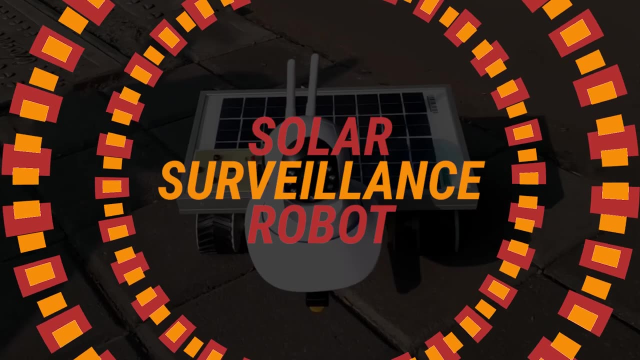 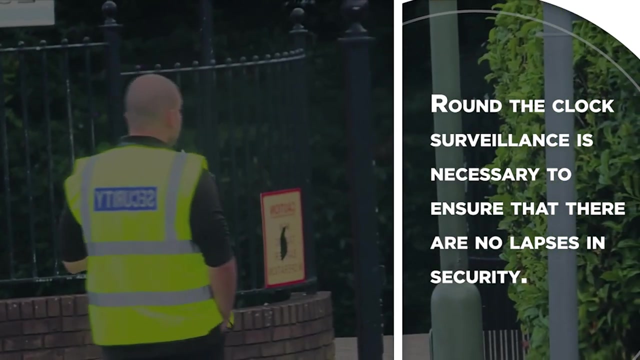 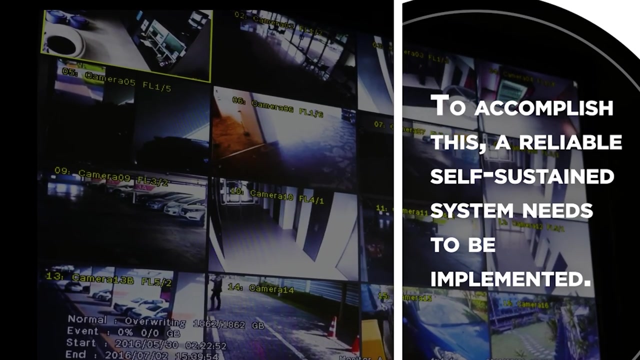 Solar Surveillance Robot. Round-the-clock surveillance is necessary to ensure that there are no lapses in security. To accomplish this, a reliable, self-sustained system needs to be implemented. So this RF-controlled solar surveillance robot can be used for cleaning and wet wiping. 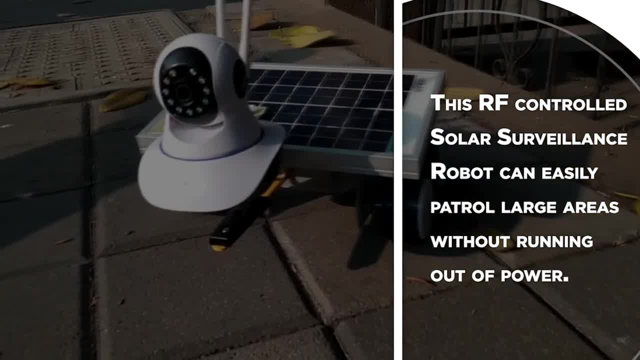 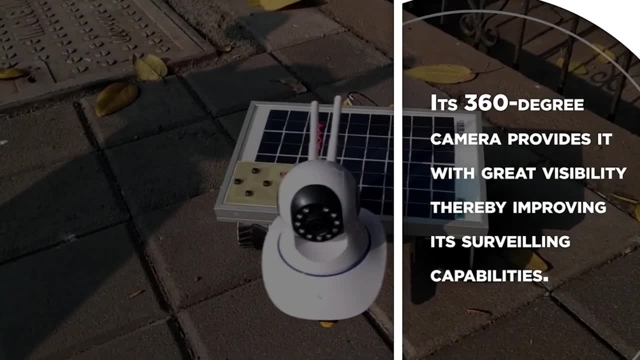 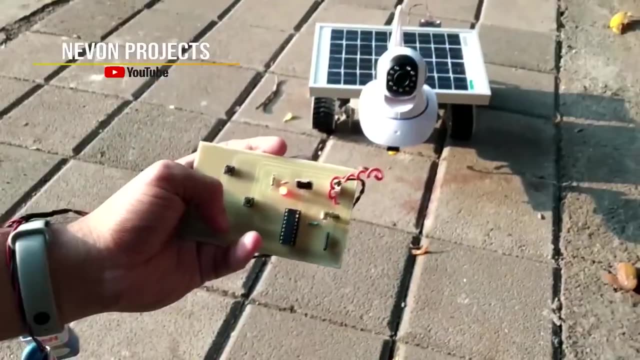 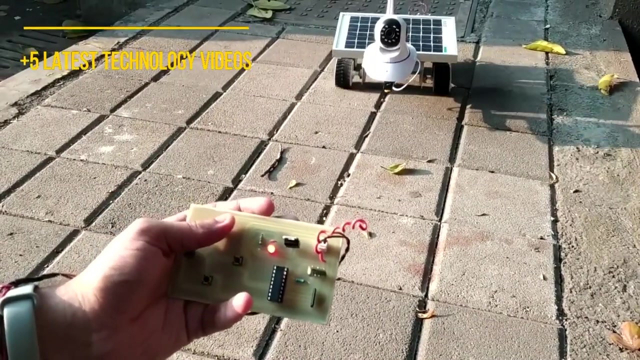 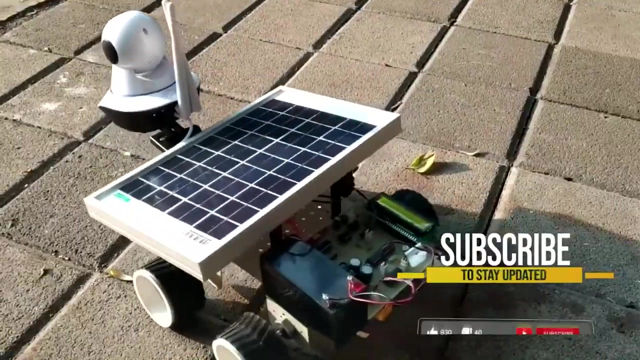 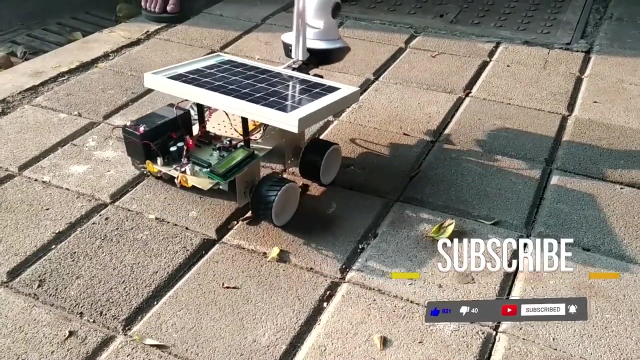 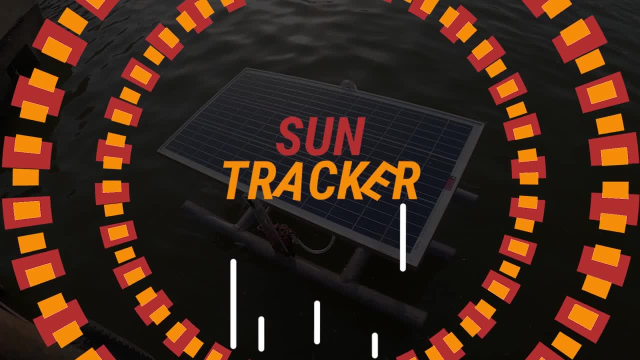 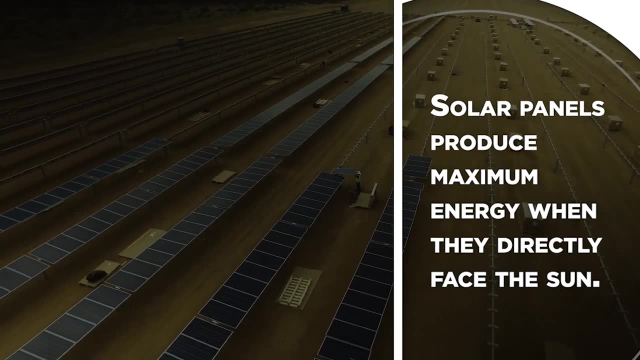 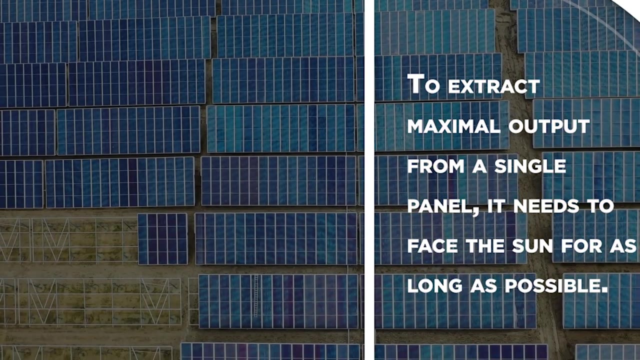 Solar Surveillance Robot can also be used for monitoring and monitoring of the environment. Floating Sun Tracker. Solar panels produce maximum energy when they directly face the sun. To extract maximal output from a single panel, it needs to face the sun. To extract maximal output from a single panel, it needs to face the sun. 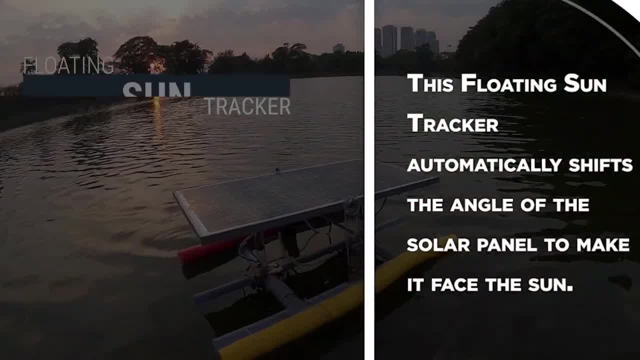 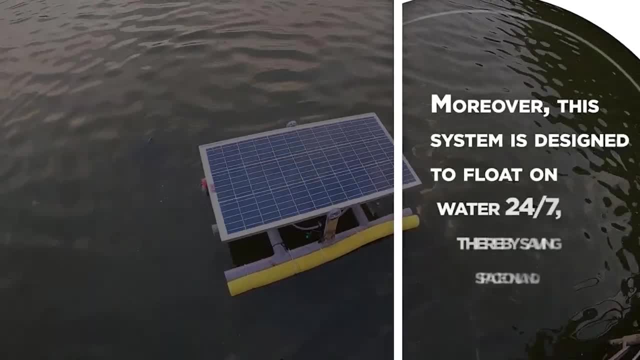 Its solar panel is capable of sending 10-20 mms of solar energy into a single panel. This floating sun tracker automatically shifts the angle of the solar panel to make it face the sun. Moreover, this system is designed to float on water 24 by 7, thereby saving space on land. 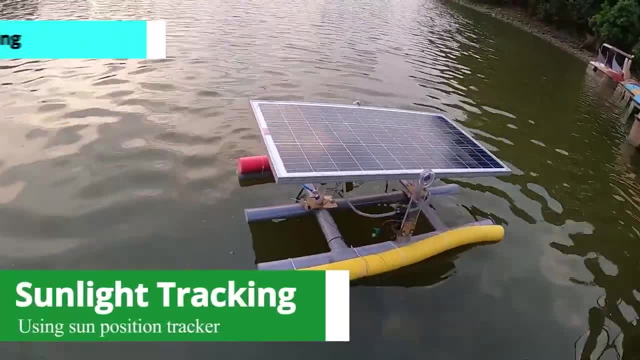 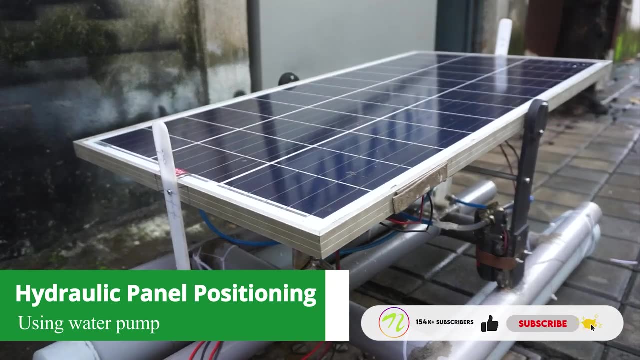 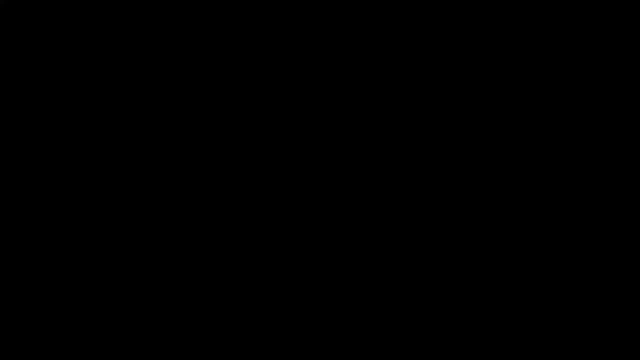 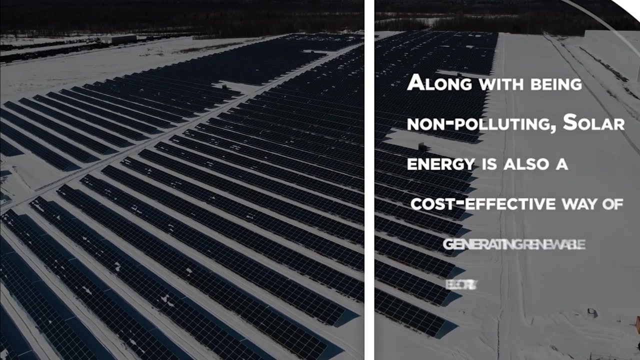 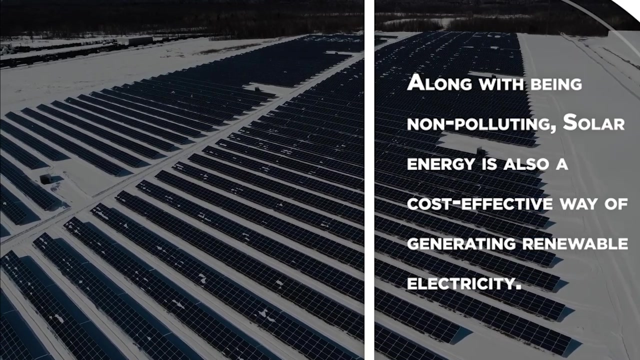 Solar panel can also produce maximum energy when it faces the sun. Solar panel can also produce maximum energy when it faces the sun. Solar Panel Cleaner Robot. Along with being non-polluting, solar energy is also a cost-effective way of generating renewable electricity. 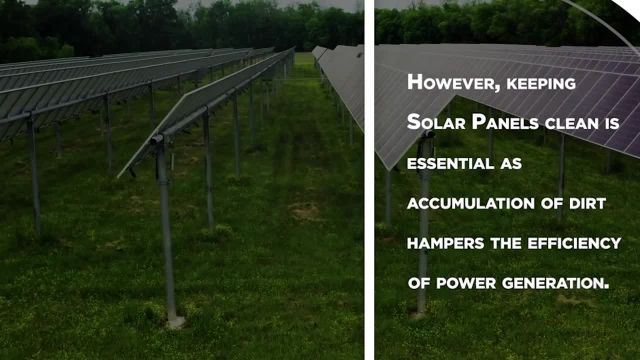 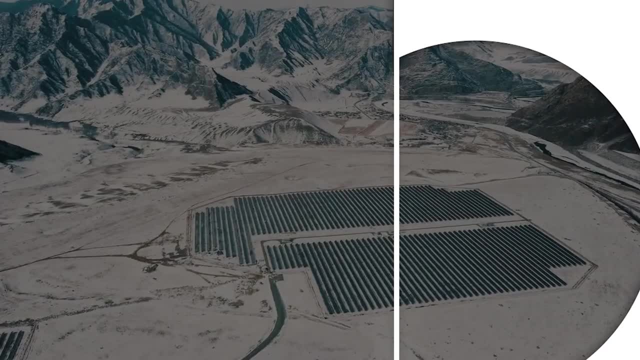 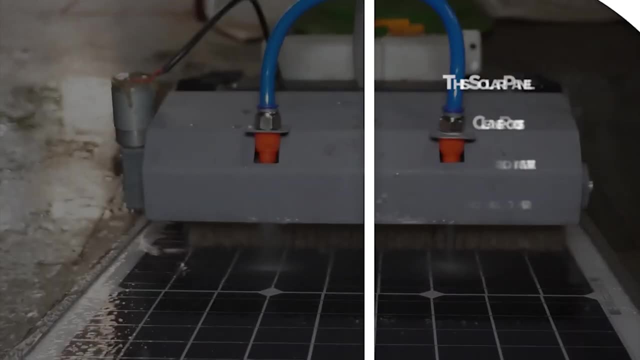 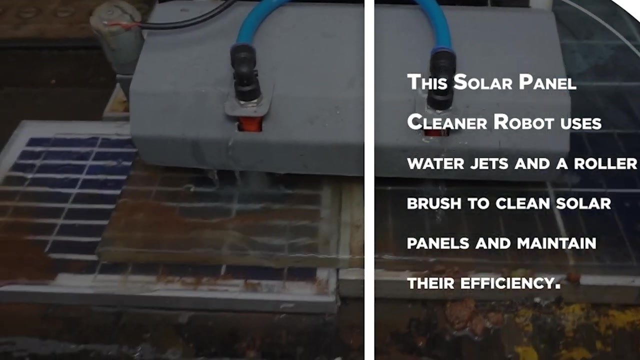 However, keeping solar panels clean is essential, as accumulation of dirt hampers the efficiency of power generation, although manually cleaning solar panels can be tedious and hazardous, So this solar panel cleaner robot uses water jets and a roller brush to clean solar panels and maintain their efficiency. 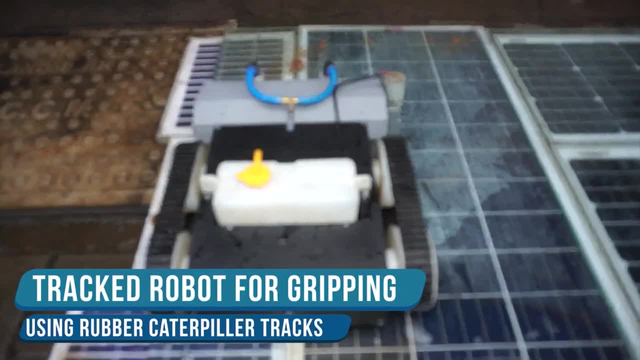 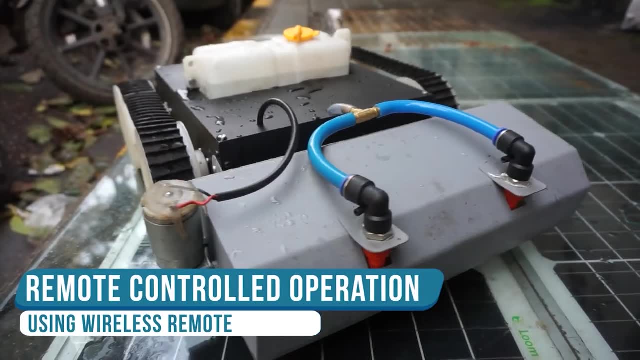 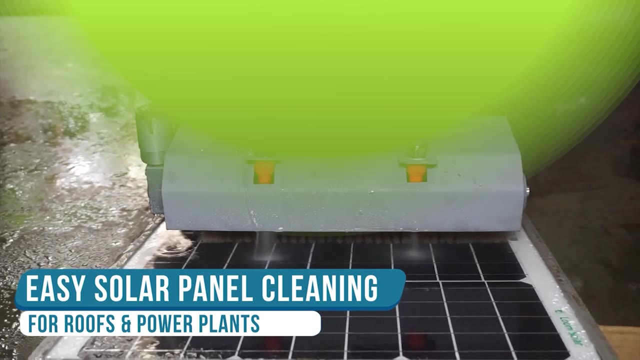 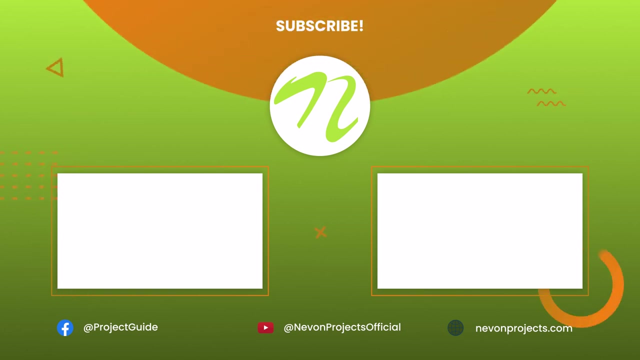 The robot is also used to clean the solar panels and clean the solar panels. The robot is also used to clean the solar panels and clean the solar panels. The robot is also used to clean the solar panels and clean the solar panels. 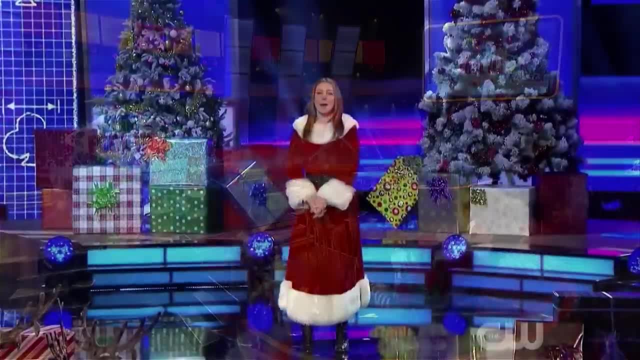 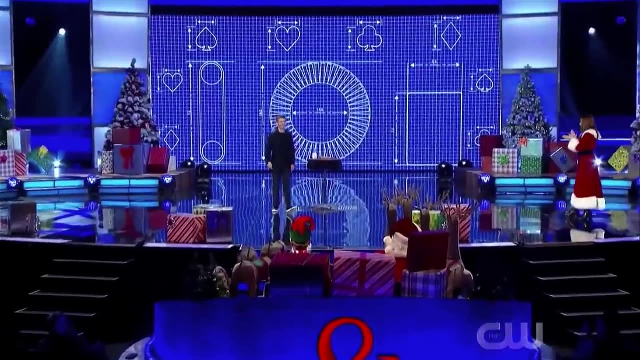 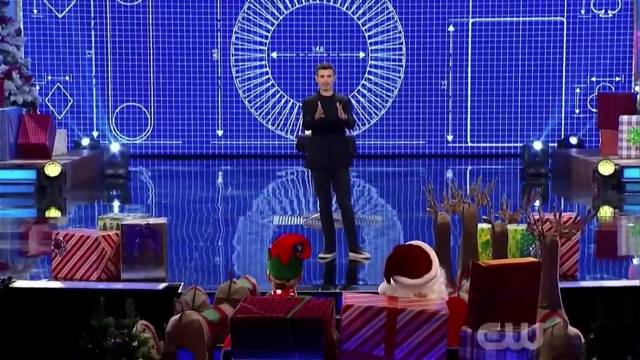 Please welcome the playful and brilliant mind of Aussie Wind. Thank you. You know every magician that's been on this show has tried to fool Penn & Teller. And then they try to figure it out and explain in code how they think it's done. 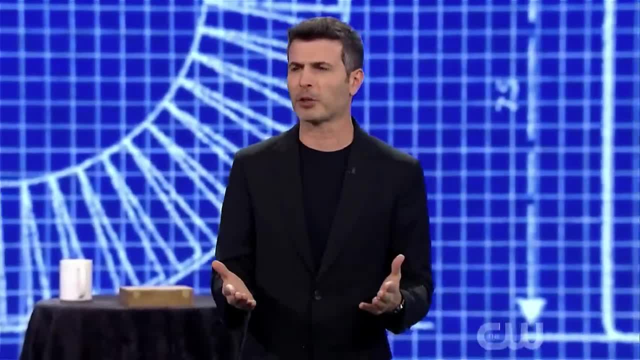 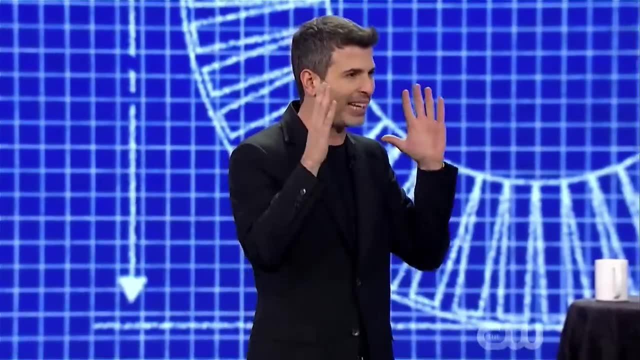 And I know what the rest of you must be thinking. You're thinking: why do they have to speak in code? That's rude. We also want to be included. We also want to know how it's done. That's why I'm going to show you a trick and explain exactly how it's done. 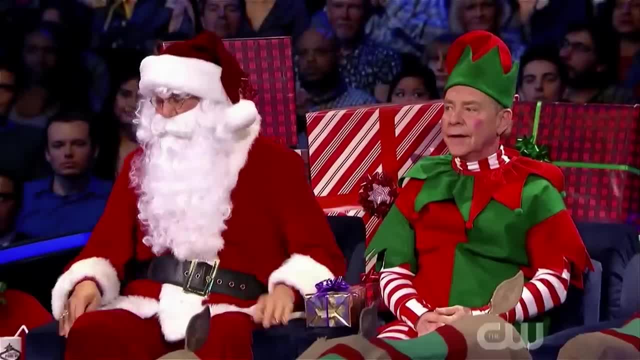 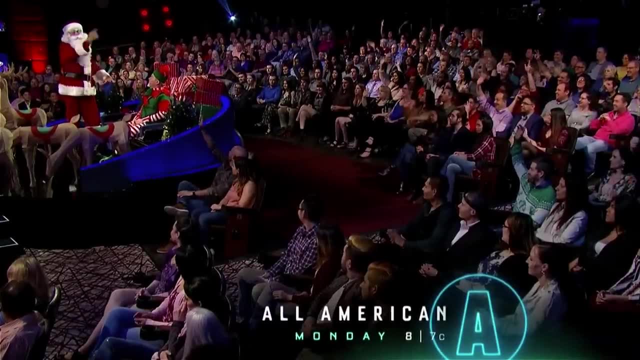 So, Penn, I need you to choose a person we can trust. Somebody from the audience- Oh, you want a regular audience person, A regular audience member Somebody. Oh, okay, Well, you got the sweater. Give me the sweater, Give me the sweater. 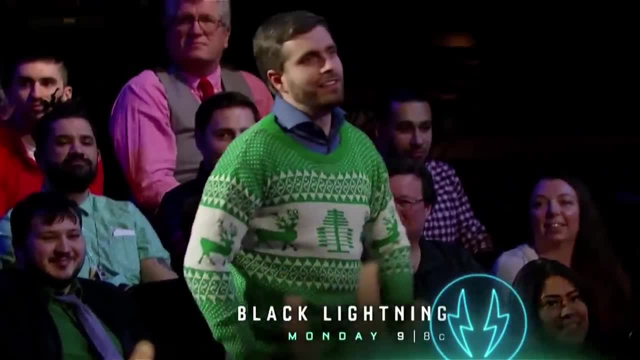 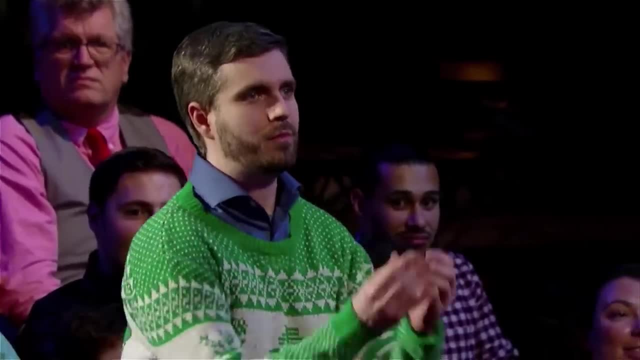 You'll seem fine, Do you mind? standing in the very spot And your name is Trevor Trevor, I want you to do me this favor. Imagine you have a deck of cards in your hands. okay, Hold them up And do you want to pull out the number cards or the picture cards? 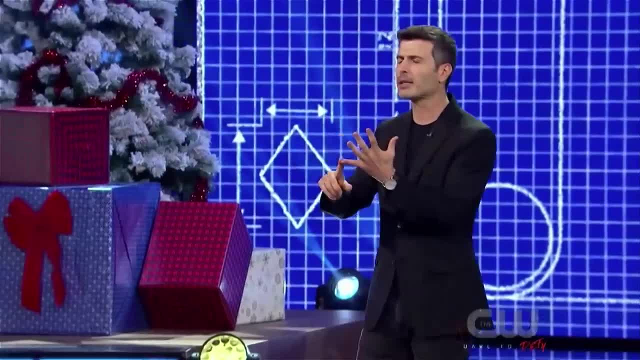 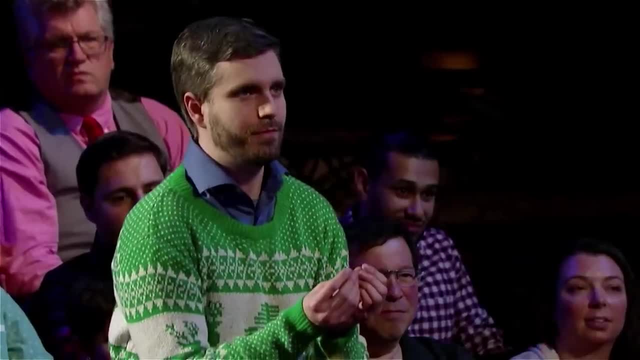 What do you want to pull out? I want to pull out the picture cards. Picture cards, That means jacks, queens and kings. Do you want jacks, queens, or kings, Kings, Oh, kings. I'll give you a few seconds to think about it, okay. 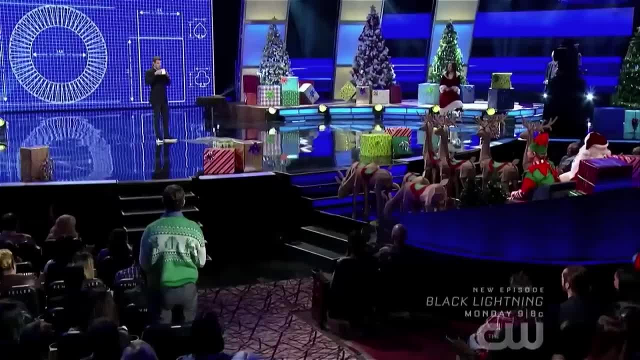 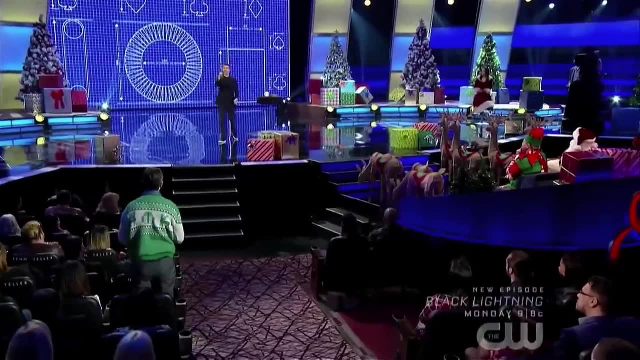 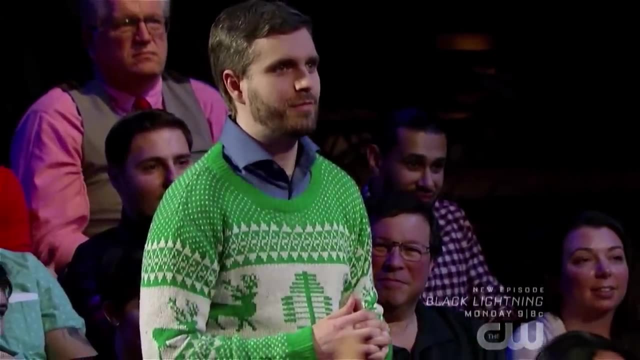 Just, you know, take your time, You don't have to rush. you know, Is it still a king? I still like kings. yeah, Kings, Hearts, clubs, diamonds or spades, Spades, The king of spades. Do you want to change your mind? one last second, You have.